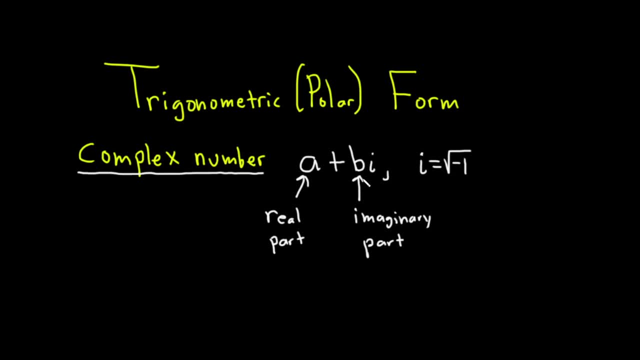 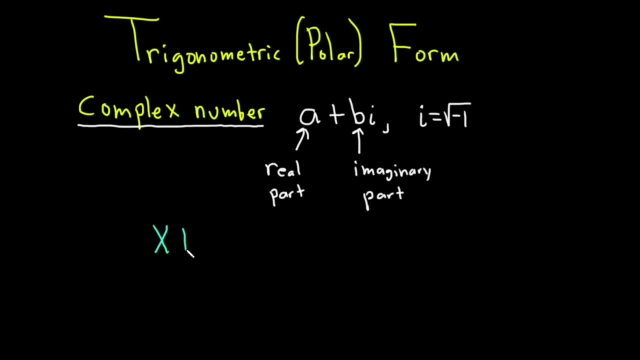 And you don't have to use a and b. In fact, you can use x and y, And so let's actually switch. just to make the point, So let's consider a complex number, x plus, And you can write it as y times i, or i times y or yi. 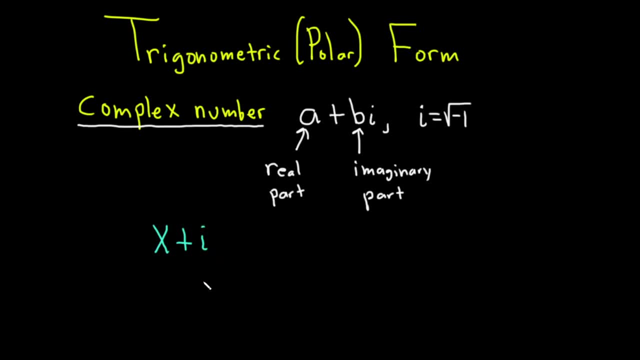 You can write it like this, Or you can write it like this: Okay, it doesn't matter how you choose to write it, I'll stick with this, just to be consistent with what's up here. Okay, so what is the trigonometric? 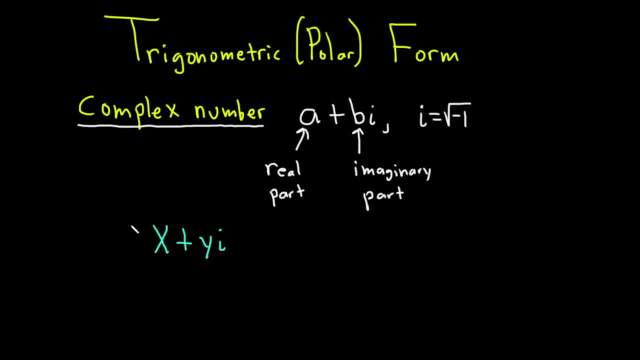 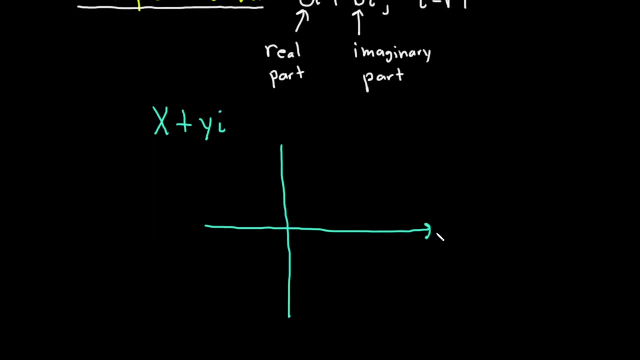 Trig form of a complex number. So let me show you. I'm going to draw a little picture here. We're going to draw the coordinate plane here, Okay, and say this is the x-axis here And this is the y-axis here. 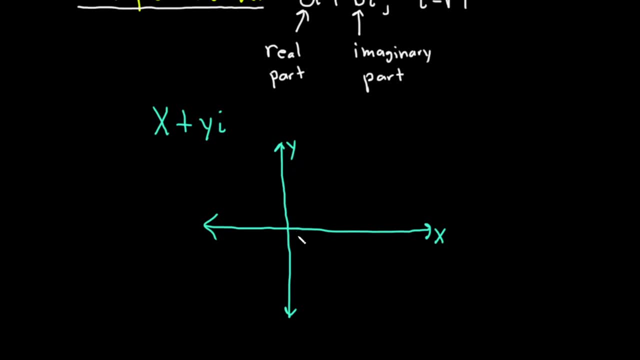 Okay, what we can do here is we can take our complex number And we can plot it, And we can plot it in the x-y plane. So you travel a distance of x- Let's say they're both positive- And a distance of y. 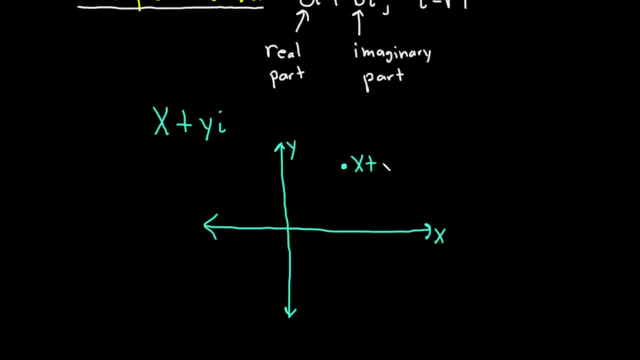 And so maybe you're here: x plus yi. Now, if this was the complex plane, this would be the real axis And this would be the imaginary axis. Okay, so we're plotting it here in the x-y plane, And now we can draw a triangle. 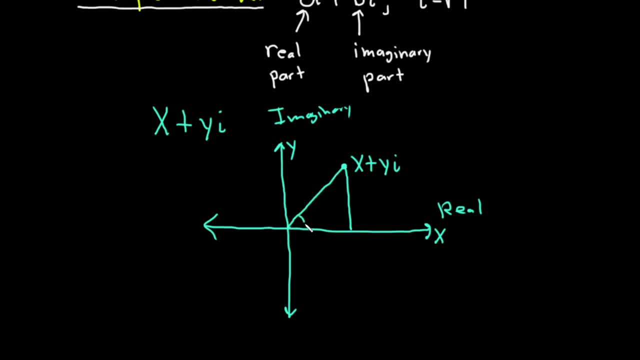 Let's do that like this, And this will be the angle theta. And this distance here is x, This distance here is y. Therefore, by the theorem of the legendary Pythagoras, I'll call this distance r, And we know that r squared is equal to x squared plus y squared. 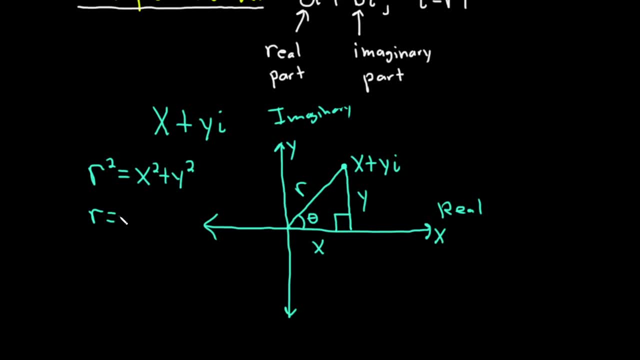 Taking the square root of both sides, we do get a plus or minus, But it's a length so it's got to be the plus. So we have this formula here for r And you can do more with this. You can create more relationships with this complex number. 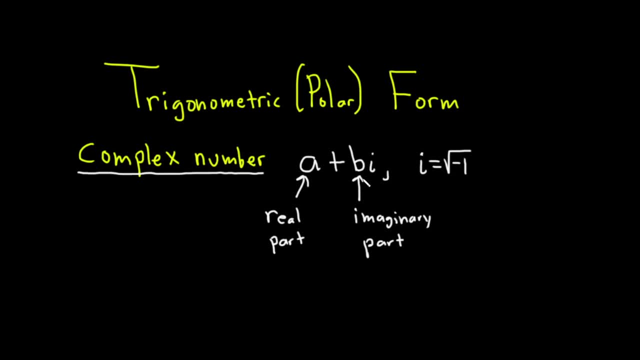 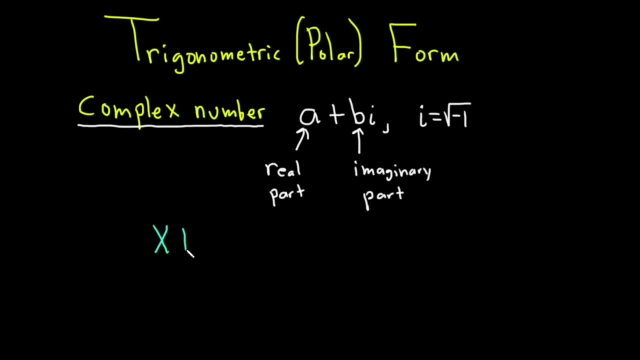 And you don't have to use a and b. In fact, you can use x and y, And so let's actually switch. just to make the point, So let's consider a complex number, x plus, And you can write it as y times i, or i times y or yi. 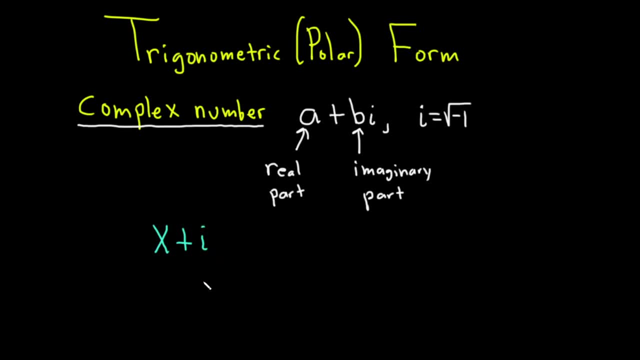 You can write it like this, Or you can write it like this: Okay, it doesn't matter how you choose to write it, I'll stick with this, just to be consistent with what's up here. Okay, so what is the trigonometric? 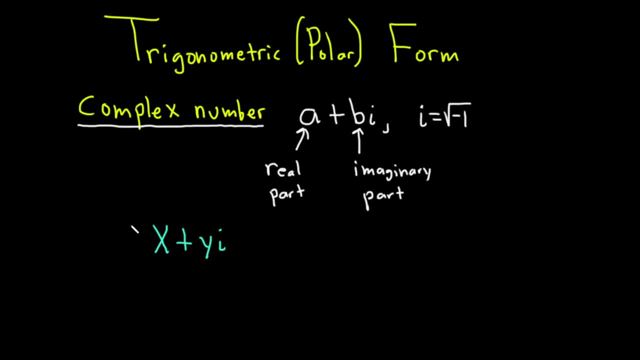 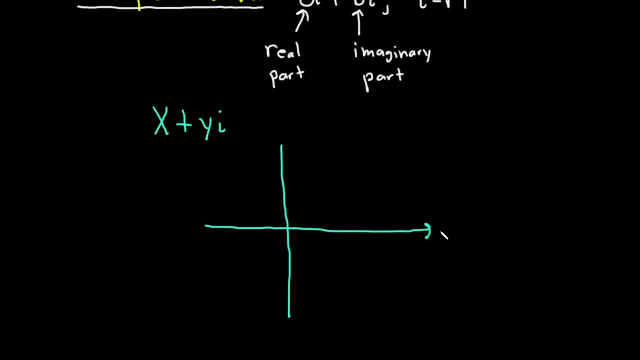 Trig form of a complex number. So let me show you. I'm going to draw a little picture here. We're going to draw the coordinate plane here, Okay, and say this is the x-axis here And this is the y-axis here. 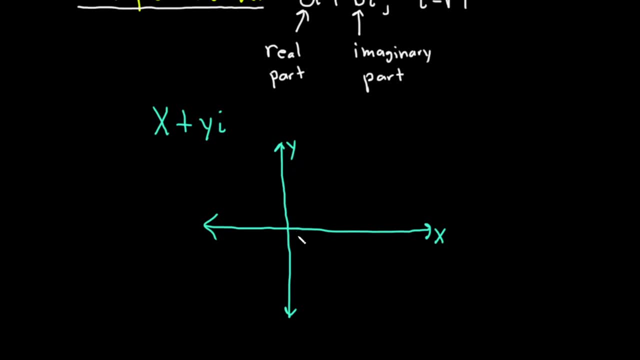 Okay, what we can do here is we can take our complex number And we can plot it, And we can plot it in the x-y plane. So you travel a distance of x- Let's say they're both positive- And a distance of y. 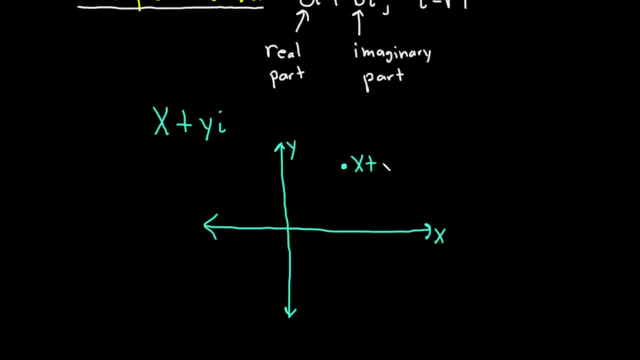 And so maybe you're here: x plus yi. Now, if this was the complex plane, this would be the real axis And this would be the imaginary axis. Okay, so we're plotting it here in the x-y plane, And now we can draw a triangle. 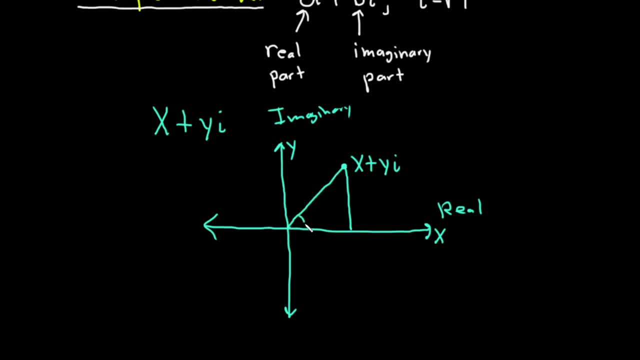 Let's do that like this, And this will be the angle theta. And this distance here is x, This distance here is y. Therefore, by the theorem of the legendary Pythagoras, I'll call this distance r, And we know that r squared is equal to x squared plus y squared. 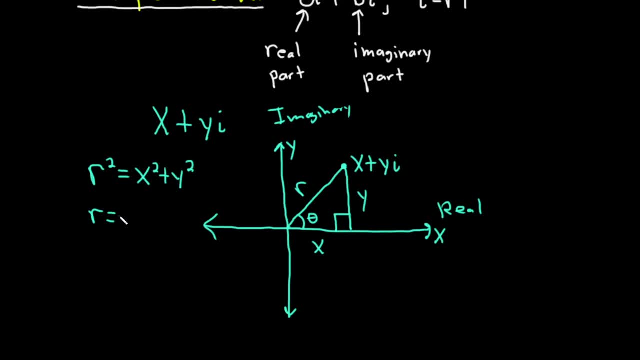 Taking the square root of both sides, we do get a plus or minus, But it's a length so it's got to be the plus. So we have this formula here for r And you can do more with this. You can create more relationships with this complex number. 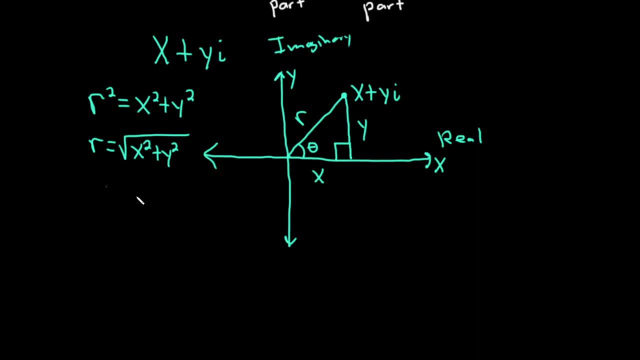 So we know r. What about x? Well, we can use SOHCAHTOA to come up with some other relationships, And I'm going to put all of this in a box in a minute, once we get there. I'm just showing you how to come up with it. 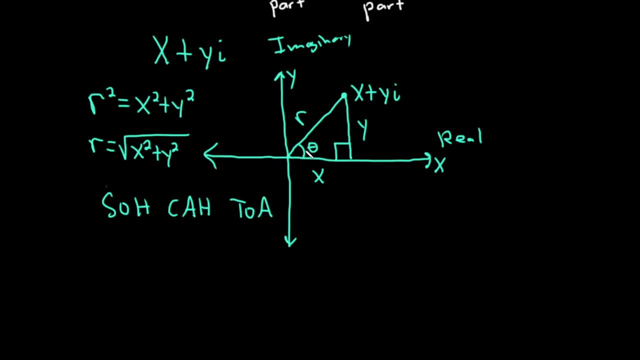 And then we'll do some examples. So sine is opposite over hypotenuse. So the sine of theta is going to be y over r. Okay, And that means that y is equal to r sine theta, Because you could multiply by r here. 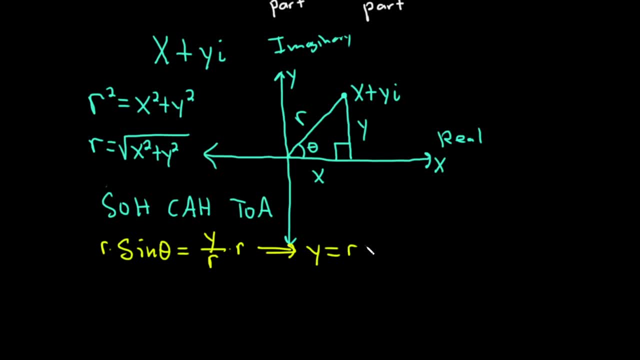 So that would give us y equals r sine theta Okay, And you can use cosine now Okay. Cosine is adjacent over hypotenuse, So the cosine of theta okay is going to be x over r, Because that's the adjacent x. 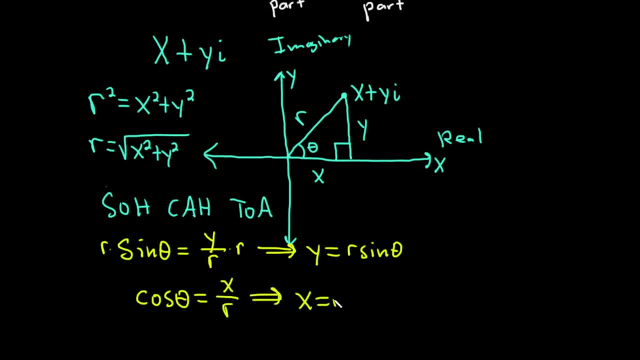 Same thing. multiplying by r gives us x equals r. Cosine theta, And you can also create a relationship for tangent, which a lot of people like to do. Tangent is opposite over adjacent, So tangent of theta would be y over x. 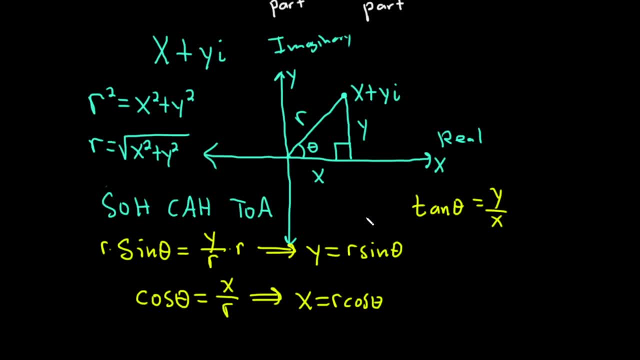 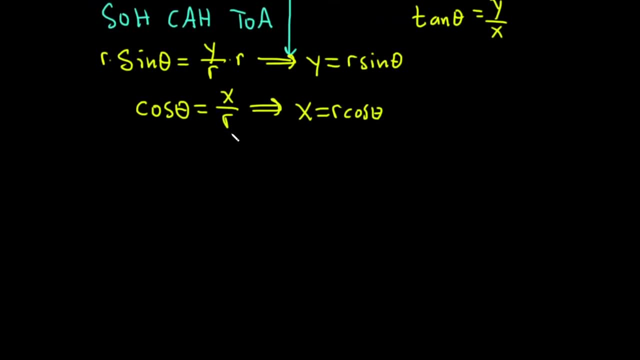 I'm going to try to avoid using the tangent function when we do the problems, And I'll talk about why. I'm going to show you a really interesting way to do these problems. So let me just give you the formulas or the relationships. 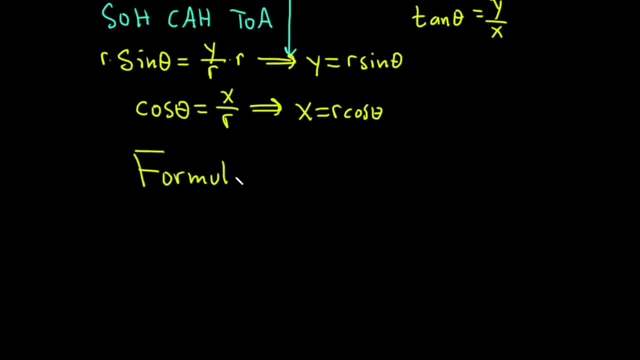 I'll just say formulas And I'm going to put them in one place Because this comes up a lot in mathematics, not just in trig. So x, we know, is r cosine theta. Okay, y is equal to r sine theta. 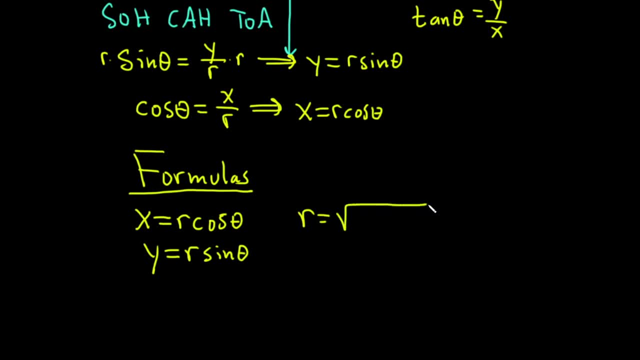 And r is equal to the square root of x squared plus y squared. Okay, And we also have this other one where tangent of theta is equal to y over x And obviously in this case, here x can't be zero. r has a name. 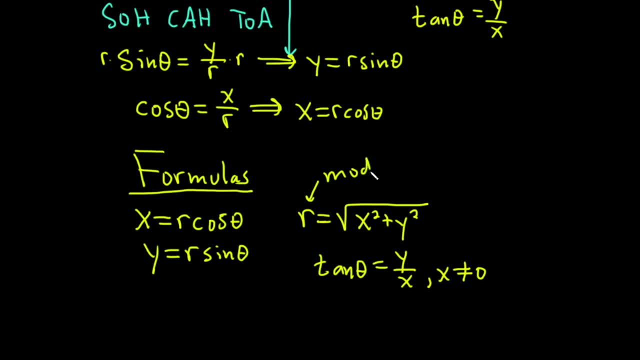 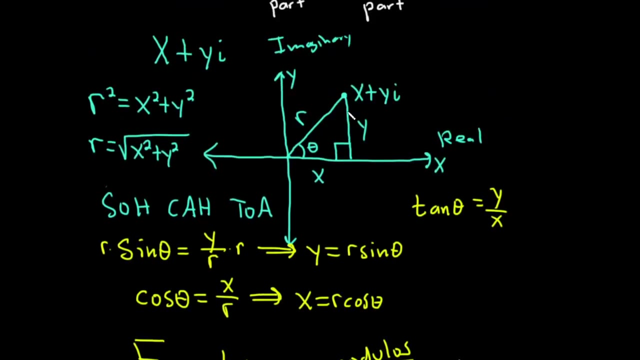 Okay, r is called the modulus of the complex number. Remember, our complex number here is x plus iy. Okay, That's our complex number. So the modulus of that would be this: If you think about it geometrically, the modulus is just the length of this vector. 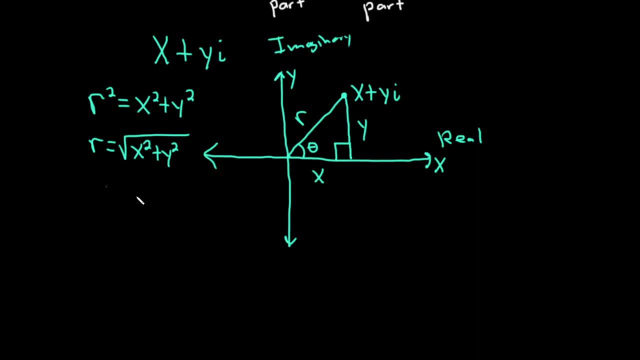 So we know r. What about x? Well, we can use SOHCAHTOA to come up with some other relationships, And I'm going to put all of this in a box in a minute, once we get there. I'm just showing you how to come up with it. 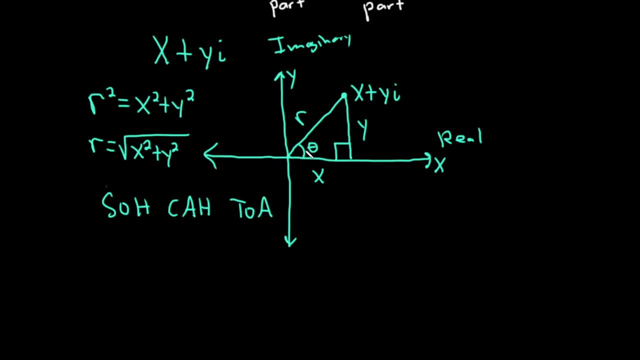 And then we'll do some examples. So sine is opposite over hypotenuse. So the sine of theta is going to be y over r. Okay, And that means that y is equal to r sine theta, Because you could multiply by r here. 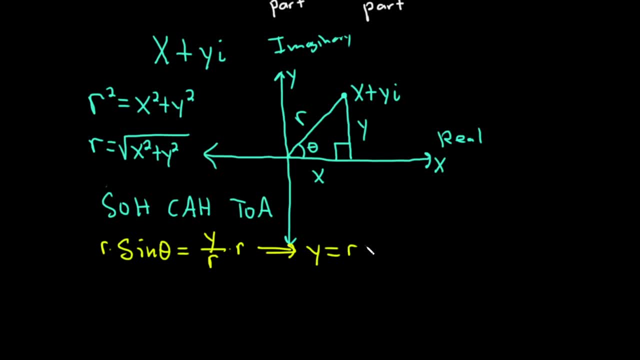 So that would give us y equals r sine theta Okay, And you can use cosine now Okay. Cosine is adjacent over hypotenuse, So the cosine of theta okay is going to be x over r, Because that's the adjacent x. 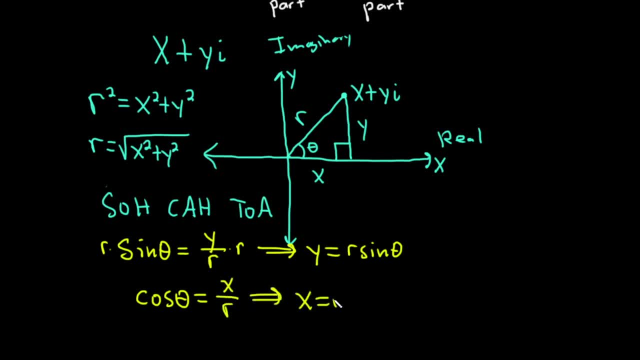 Same thing. multiplying by r gives us x equals r. Cosine theta, And you can also create a relationship for tangent, which a lot of people like to do. Tangent is opposite over adjacent, So tangent of theta would be y over x. 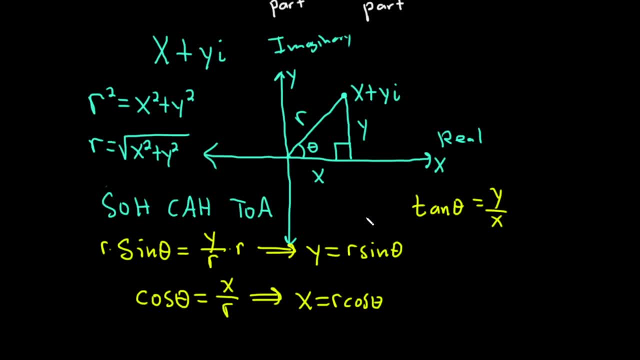 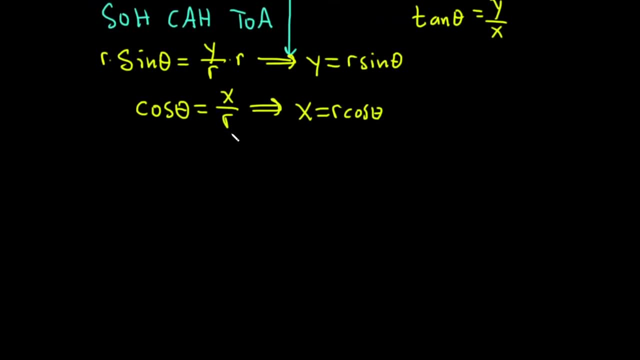 I'm going to try to avoid using the tangent function when we do the problems, And I'll talk about why. I'm going to show you a really interesting way to do these problems. So let me just give you the formulas or the relationships. 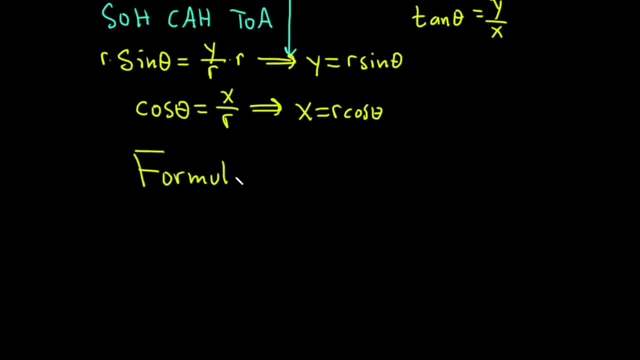 I'll just say formulas And I'm going to put them in one place Because this comes up a lot in mathematics, not just in trig. So x, we know, is r cosine theta. Okay, y is equal to r sine theta. 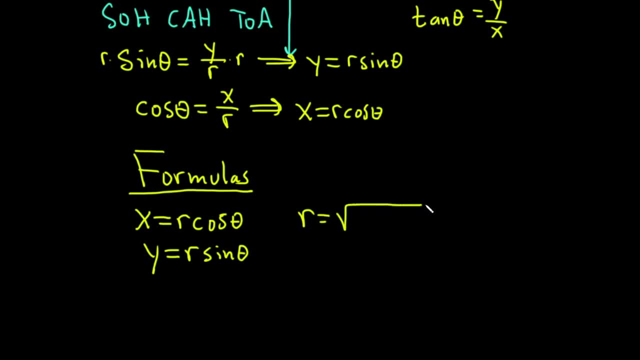 And r is equal to the square root of x squared plus y squared. Okay, And we also have this other one where tangent of theta is equal to y over x And obviously in this case here x can't be 0.. r has a name. 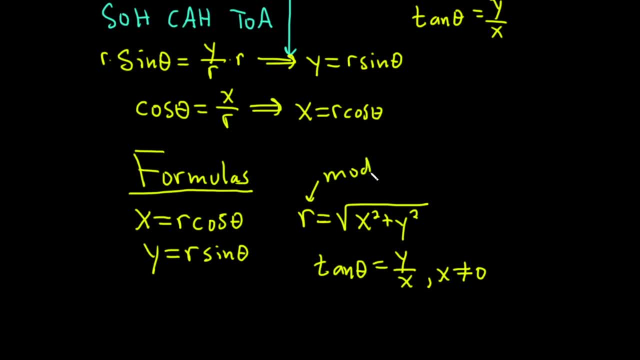 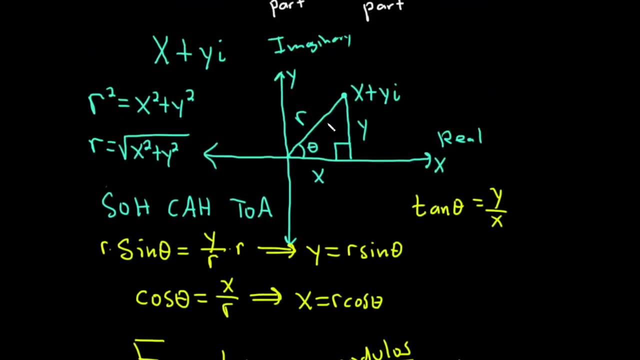 Okay, r is called the modulus of the complex number. Remember, our complex number here is x plus iy. Okay, That's our complex number. So the modulus of that would be this. If you think about it geometrically, the modulus is just. 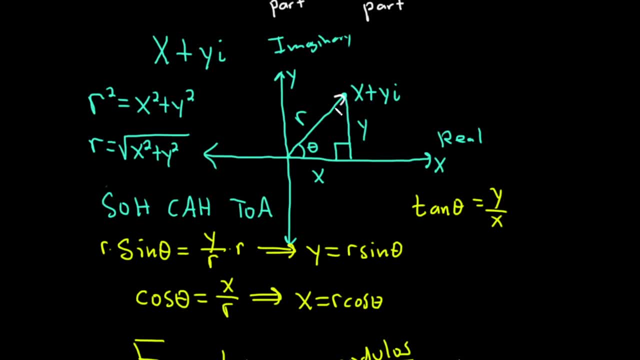 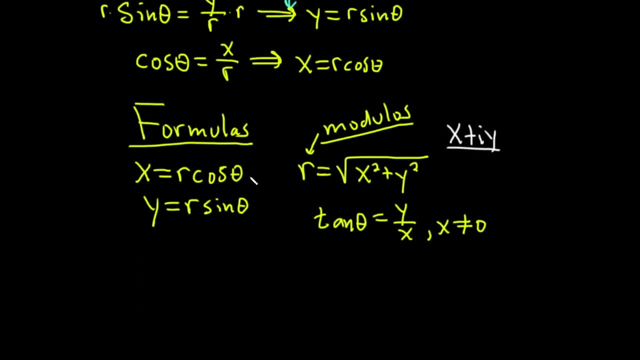 It's just the length of this vector. So if you think of this as a vector, it would be the length of this vector. Okay, That's the modulus, Pretty cool. So the magnitude of the vector: right Created of the vector, with endpoint being a complex number. 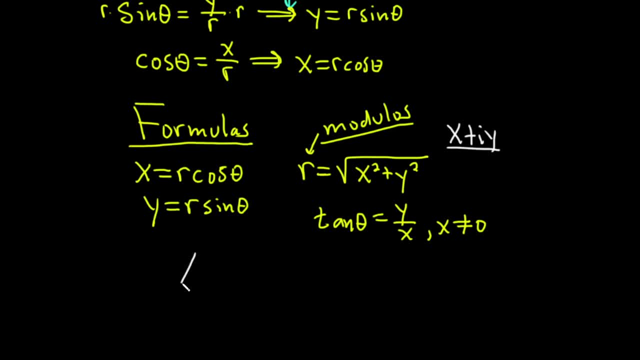 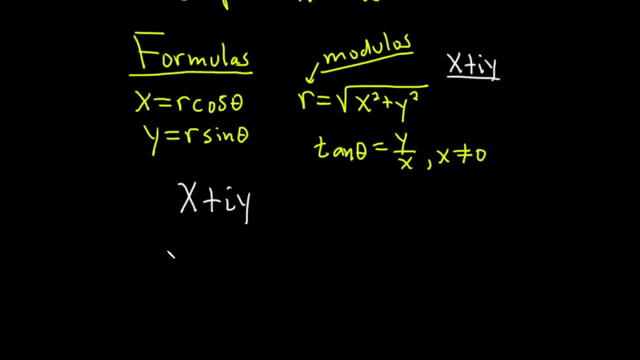 So what you can do now is we have x plus iy, And so what is the trig form? So basically you replace it with these formulas: So x is r cosine theta Plus i, And then y is r sine theta. 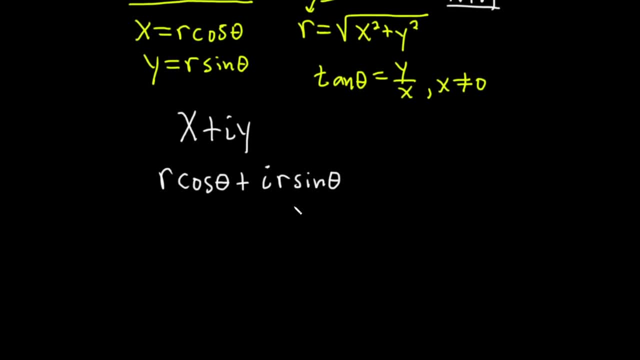 And then you can pull out the r. Okay, You can factor it out So you'll get r, parentheses cosine theta plus i sine theta. Okay, Pretty cool, Pretty cool. Some people give this a name, So some textbooks they call this. 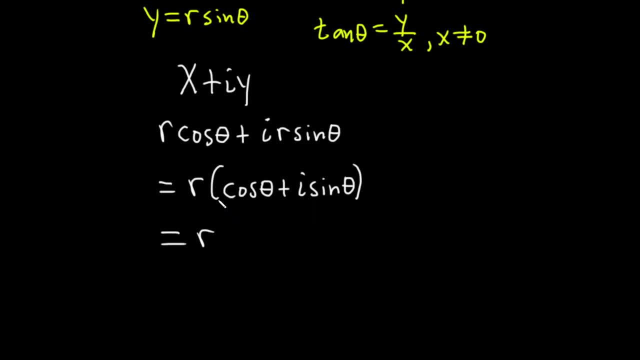 So they'll do this. They'll say: r is This is rather, This is cis theta. Let's see What's cis theta. This, This is cis theta. Cis stands for cosine i sine. You see, cosine i sine. 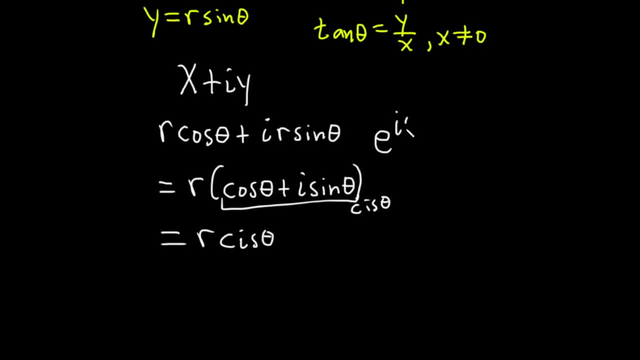 Another way to do it is to know that e to the i theta is the same thing as cosine theta plus i sine theta. So later on, if you study more mathematics, this is how you'll see it. Okay, So that's often introduced in trigonometry books and trigonometry classes that you take. 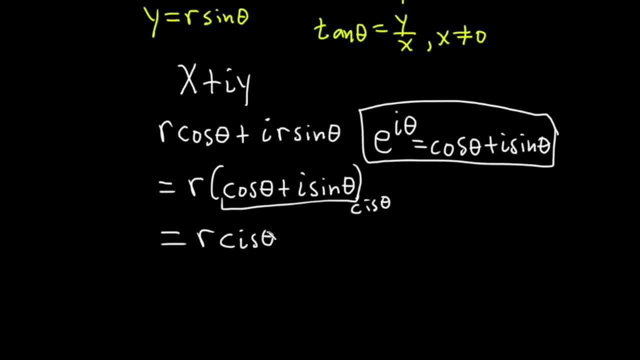 whether they be in high school or college, as a little acronym to help you memorize it. But I personally think this is cooler. But cis works too. It helps you memorize it. Cosine i sine, Cosine i sine. It's pretty easy to memorize, honestly, and you probably will. 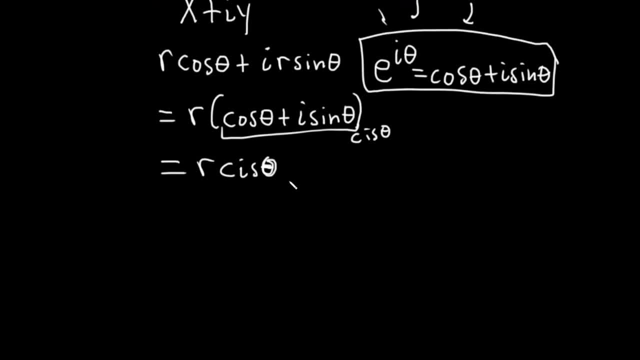 Theta. We should say something about theta here. So for our purposes we're going to specify theta, at least for this particular video We're going to say theta is between 2 pi and 0. That's if we're in radians. 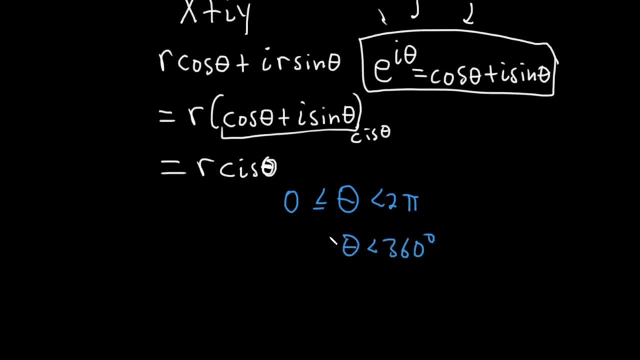 Obviously, if we're in degrees, we'll say it's between 360 degrees and 0 degrees. We'll include the 0. We'll exclude this other endpoint. This is called the argument, So theta is called the argument, The argument of the complex number. 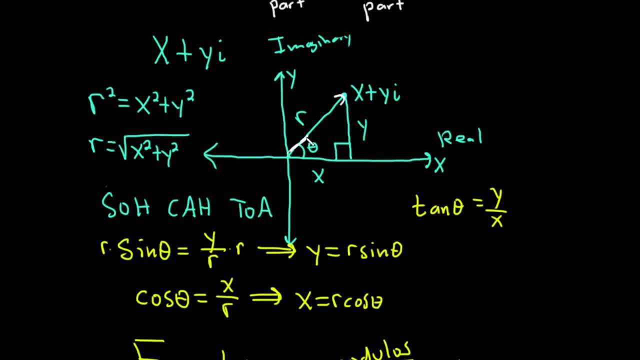 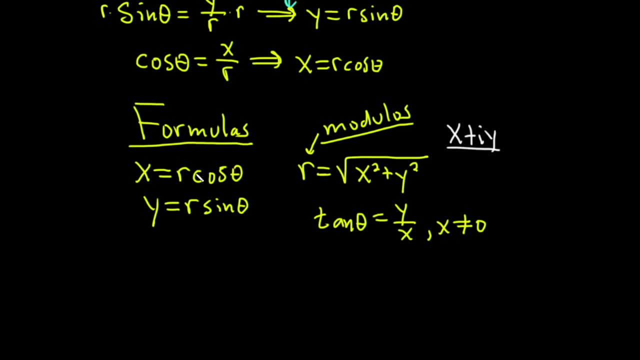 So if you think of this as a vector, it would be the length of this vector. Okay, That's the modulus, Pretty cool. So the magnitude of the vector, right created of the vector, with end point being a complex number. 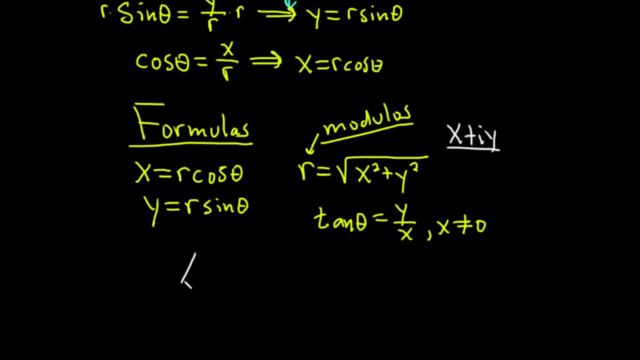 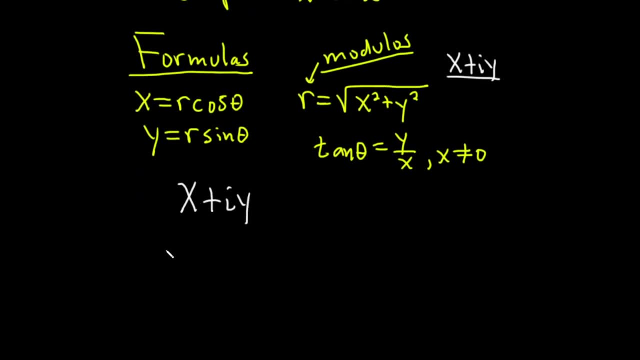 So what you can do now is we have x plus iy, And so what is the trig form? So basically you replace it with these formulas: So x is r cosine Theta plus i, and then y is r sine theta, and then you can pull out the r. 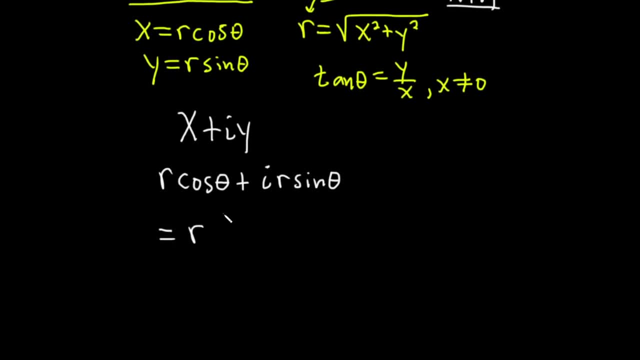 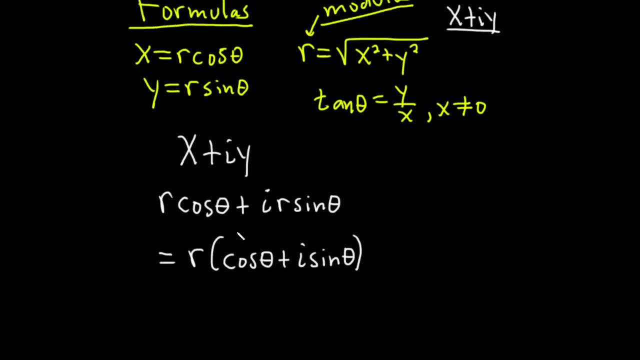 Okay, You can factor it out, So you'll get r parentheses, cosine theta plus i sine theta. Okay, Pretty cool. Pretty cool. Some people give this a name, So some textbooks they call this Um, so they'll do it. 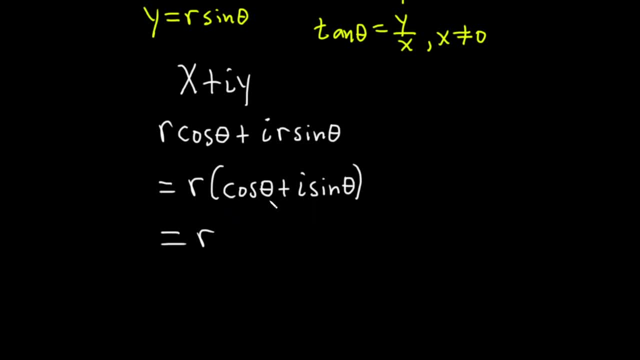 They'll do it, They'll do this. They'll say: r is uh, this is, rather, this is cis theta. Let's say: what's cis theta? This, This is cis theta. Uh, cis stands for cosine i sine. 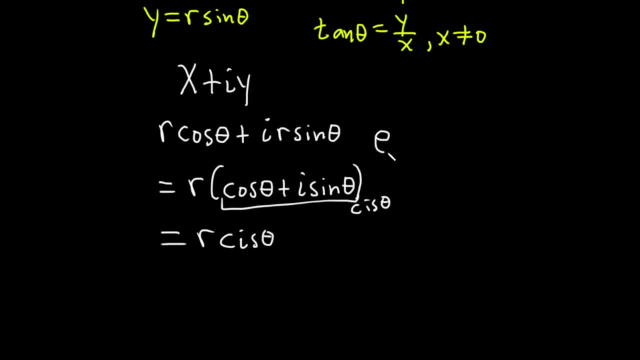 You see, cosine i sine. Uh, another way to do it is to know that e to the i theta is the same thing as cosine theta plus i sine theta. So later on, if you study more mathematics, um, this is, this is how you'll see it. 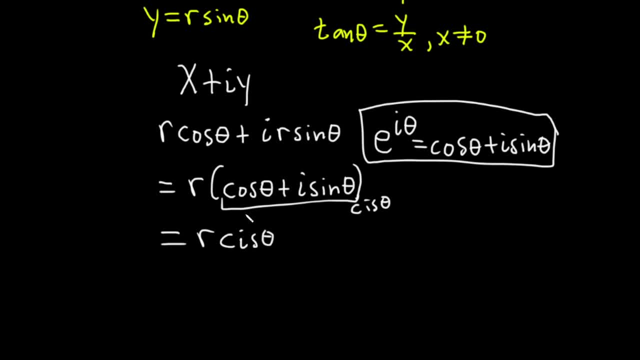 Okay, So cis theta is something that's Often introduced in trigonometry books and trigonometry classes that you take, whether they be in high school or college. um, as a little acronym to help you memorize it. But um, I personally think this is cooler. but cis works too. 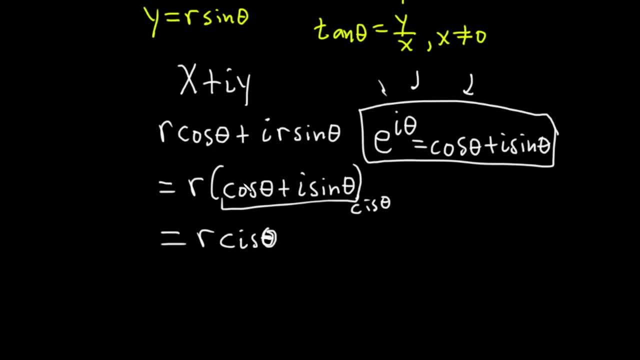 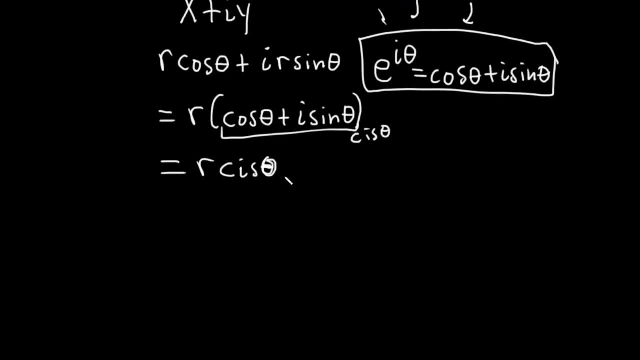 It helps you memorize it: Cosine i sine, cosine i sine. It's pretty easy to memorize, honestly, and you probably will. Um theta, we should say something about theta here. So for our purposes we're going to specify theta, at least for this particular video. 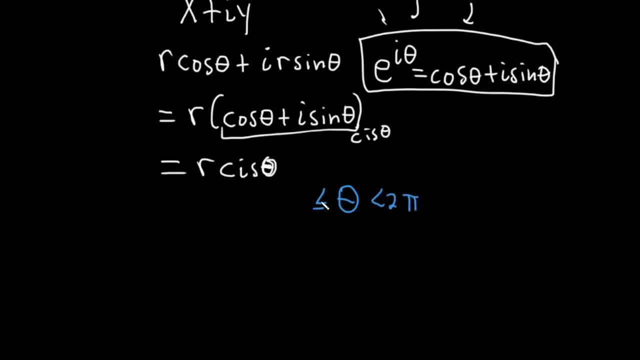 We're going to say theta is between two pi and zero, That's if we're in radians, Obviously. if we're in degrees, we'll say it's between 360 degrees and zero degrees. We'll include the zero. We'll exclude this other endpoint. 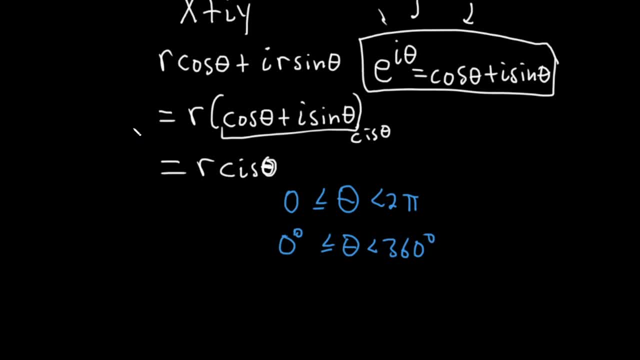 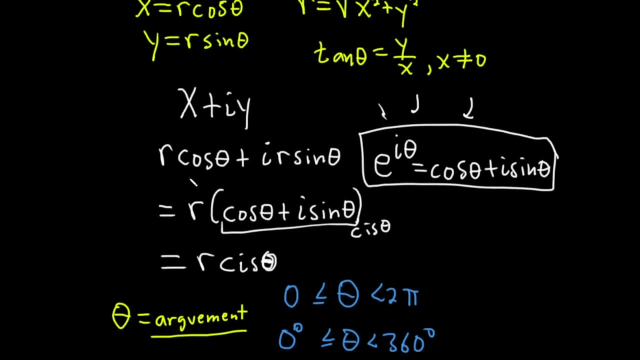 Um, this is called the argument. So theta is called the argument, The argument of the complex number. Okay, So all kinds of of stuff, right, And remember, R is the modulus. So basically a complex number can be written as the modulus times cosine of theta plus i, sine theta, where theta is the argument. 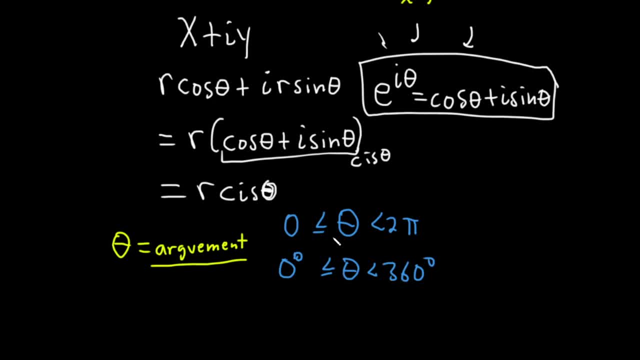 Different textbooks give different restrictions on this. So again, if you go further in math, always read the book that you're reading. A common one would be from negative pi to pi. Um, let's, let's go ahead and just uh, maybe do uh. a simple example. 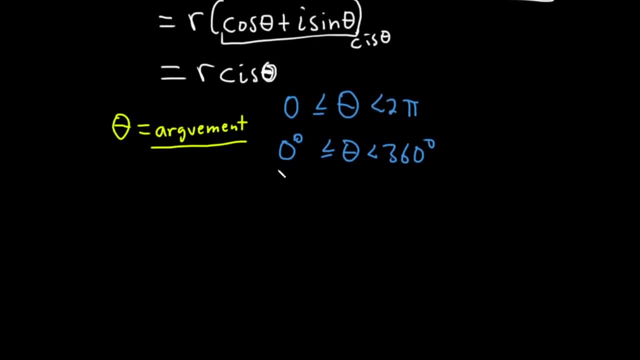 Uh, and this is actually not an easy example, We're going to do a harder one, Uh, and then in the videos that follow, you'll see, uh, lots of examples, uh, of going to polar form. Harder examples as well. 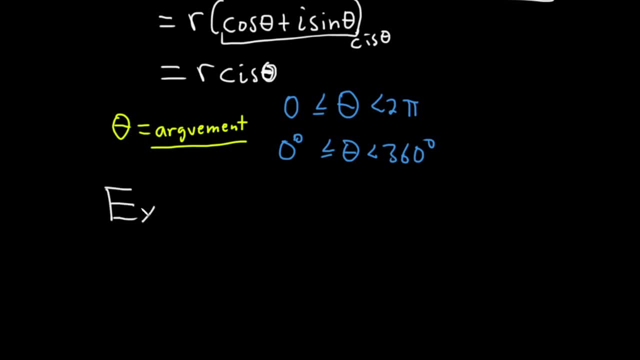 But let's start with one here And again. this is not one that's particularly easy, And I'm going to do it, uh, a little bit different than most people do. I'm going to show you how to do it. So, basically, we have this complex number negative root three plus i. 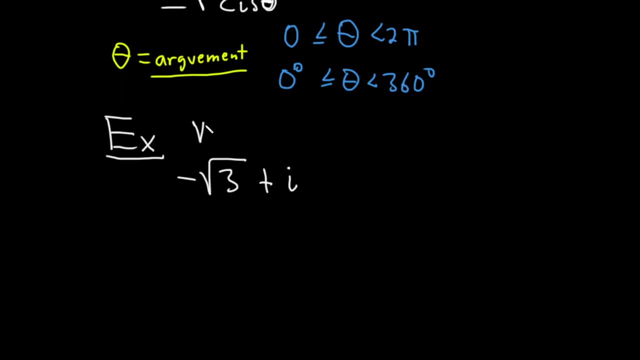 And we're going to write this in trig form or in polar form. So write, write in trig form, which is the same thing as as polar, Or in polar form. Okay, So I always start by drawing a little picture, or at least you know, being aware of where it is. 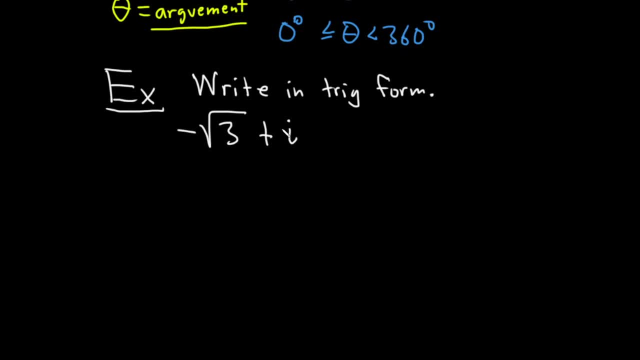 So this complex number? where is it? Um well, if you're having a problem with the i, you can think of the complex number as an ordered pair: Negative root, three comma and the coefficient of the i. here is a one here. 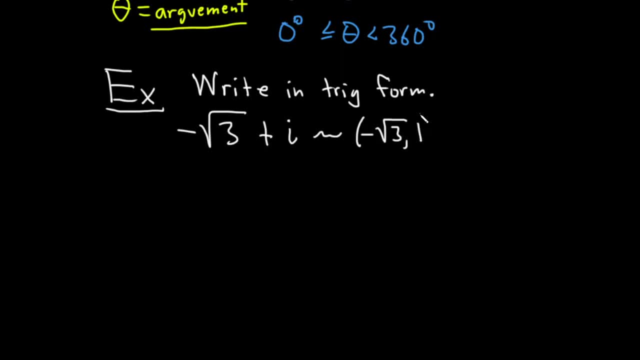 Right, There's really an invisible one, So one. So where's that going to be? That's going to be over here, right, Left three Down one. So over here somewhere. So we're going to be down here, uh, in quadrant, uh, oh no, that's, that's a plus one. 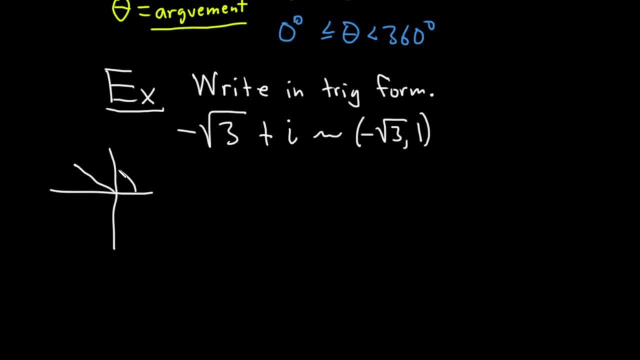 My picture's off. We're going to be here in quadrant two. For some reason I was thinking it was a negative. So we're here in quadrant two, Right Left, uh, square root of three up one, and that puts us right here. 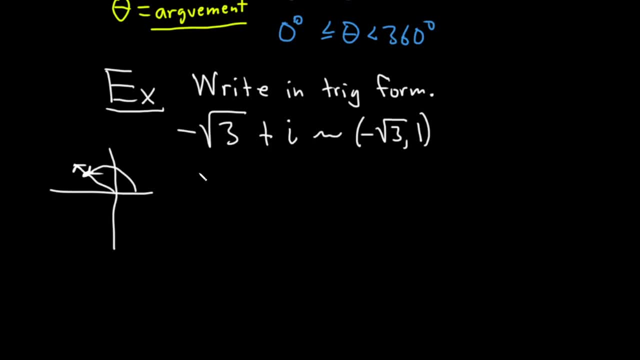 Okay, That's really important to know where you are. So, uh, we're going to come back to that later. The next thing I like to do in these problems is find- Find the modulus. So there is a one here. 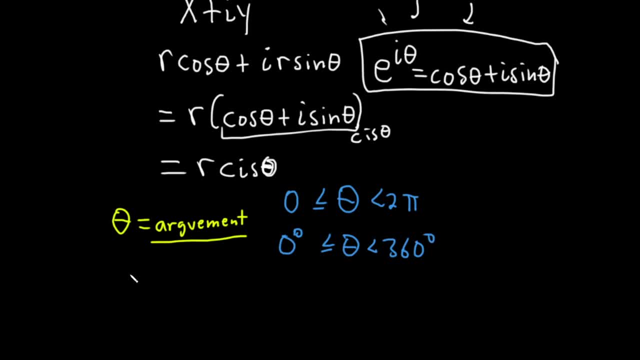 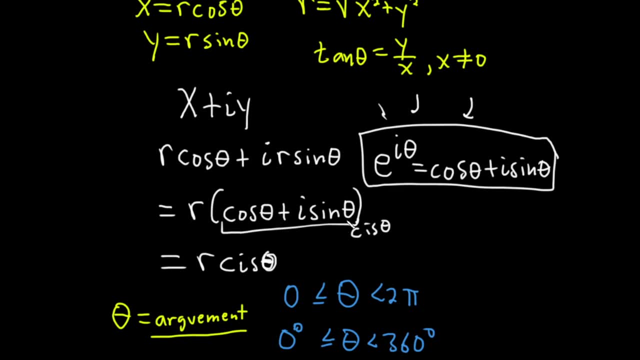 So all kinds of stuff right. And remember, r is the modulus. So basically a complex number can be written as the modulus times cosine of theta plus i sine theta, where theta is the argument. Different textbooks give different restrictions on this. 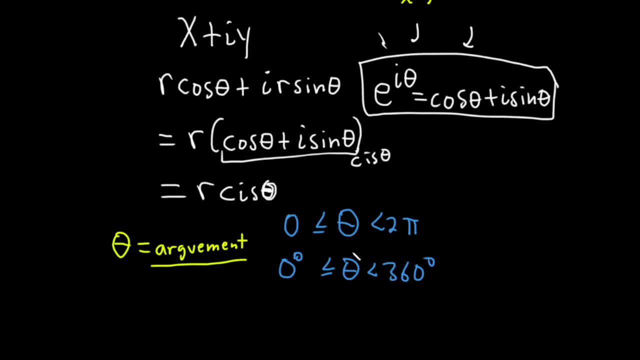 So again, if you go further in math, always read the book that you're reading. A common one would be from negative pi to pi. Let's go ahead and just maybe do a simple example, And this is actually not an easy example. 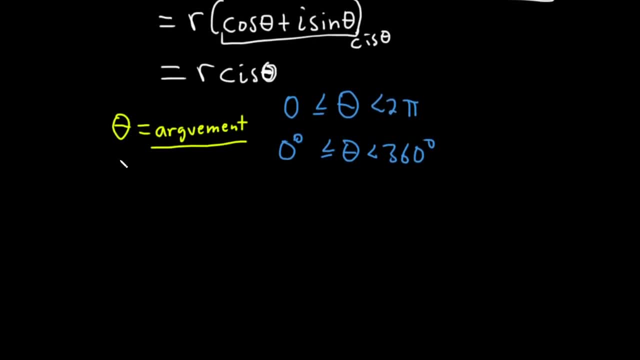 We're going to do a harder one, And then, in the videos that follow, you'll see lots of examples of going to polar form- harder examples as well, But let's start with one. here And again, this is not one that's particularly easy. 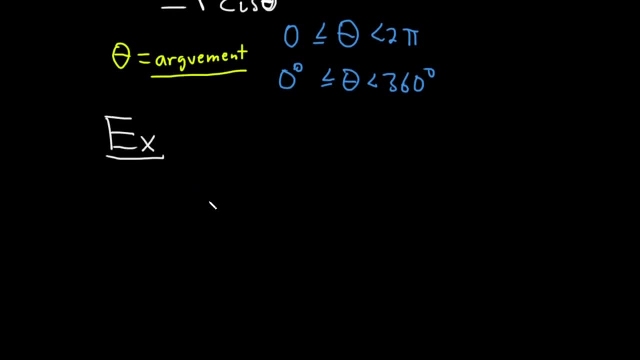 And I'm going to do it a little bit different than most people do. I'm going to show you how to do it. So, basically, we have this complex number, negative root 3 plus i, And we're going to write this in trig form or in polar form. 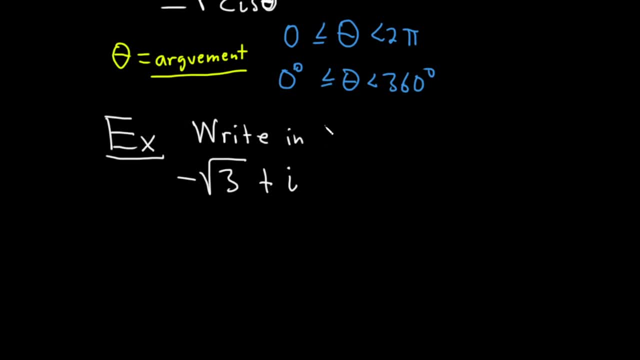 So write, Write in trig form, which is the same thing as polar form. So I always start by drawing a little picture, or at least being aware of where it is. So, this complex number, where is it? Well, if you're having a problem with the i, you can think of the complex number as an ordered pair. 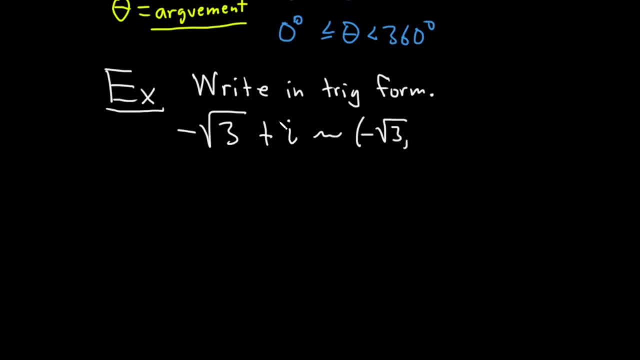 Negative root, 3, comma, and the coefficient of the i. here is a 1, here There's really an invisible 1.. So 1.. So where is that going to be? That's going to be over here, right? 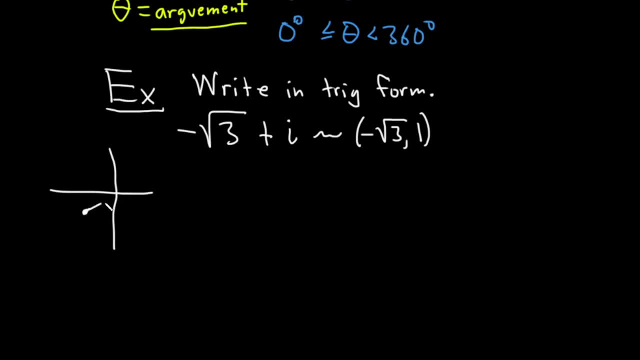 Left 3, down: 1. So over here somewhere. So we're going to be down here in quadrant. Oh no, That's a plus 1. My picture is off. We're going to be here in quadrant 2.. 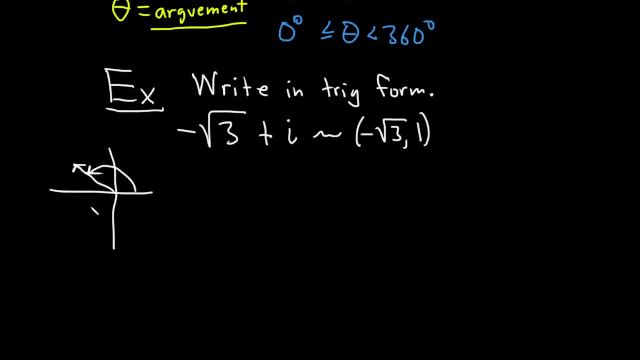 For some reason I was thinking it was a negative. So we're here in quadrant 2.. Right, Left, square root of 3, up 1.. And that puts us right here. Okay, That's really important to know where you are. 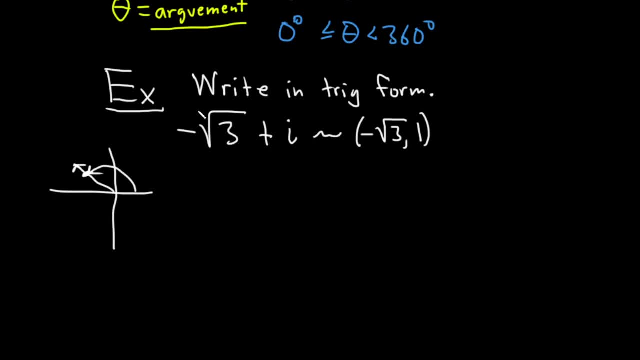 So we're going to come back to that later. The next thing I like to do in these problems is find the modulus. So there is a 1 here, So r is equal to the square root of So x. here, by the way, is negative root 3.. 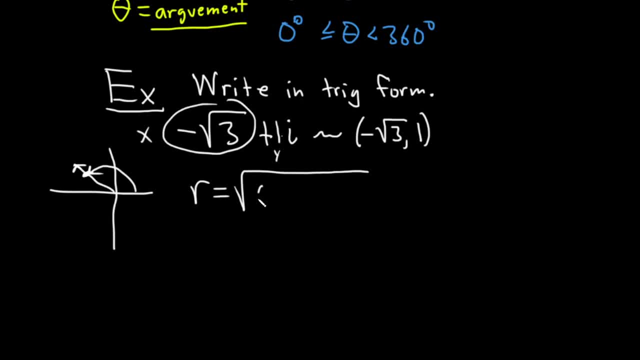 And then y is equal to 1.. Okay, This will be negative root: 3 squared plus 1 squared. This is going to be the square root of When you square this. you're just going to get 3.. Square 1,, you get 1.. 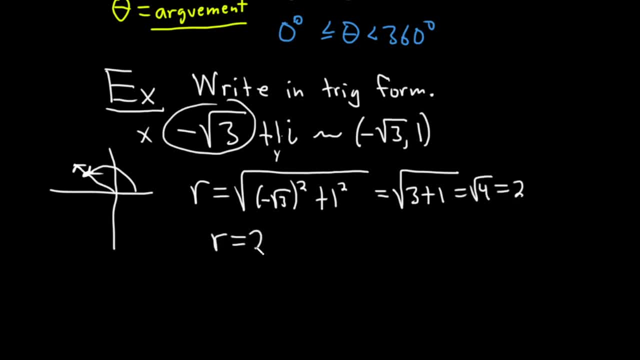 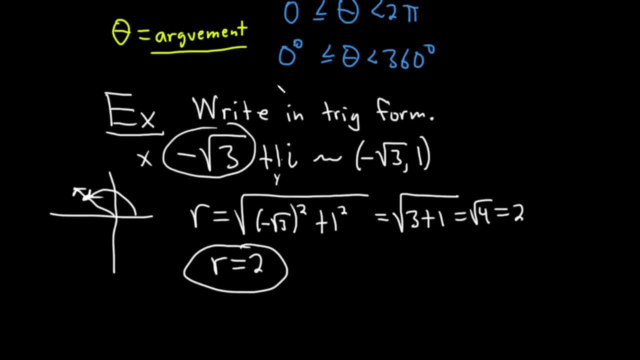 Get the square root of 4.. So you get 2.. So r is 2., So r is 2.. Okay, That's the modulus Most people. what they do now is they look at the tangent function and they do. tan of theta equals y over x. 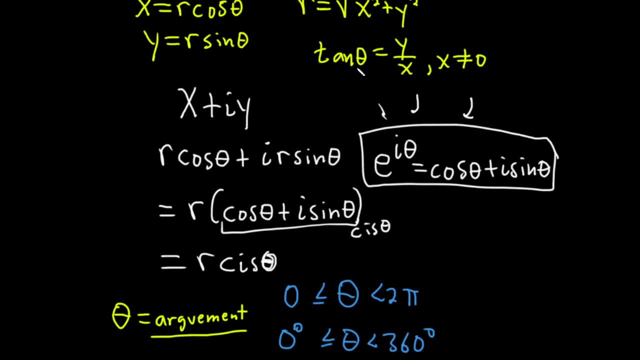 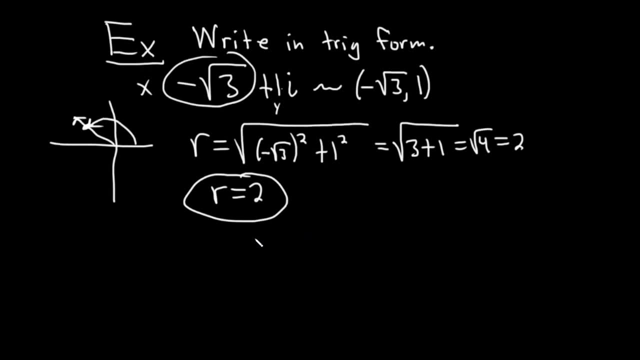 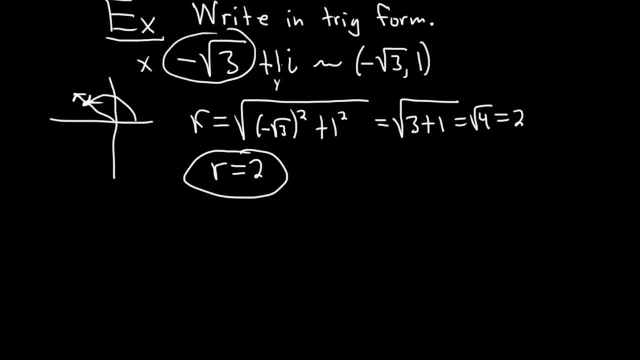 You could do that, but maybe you don't have, you know, the trig function, values of the tangent function memorized. In fact a lot of people don't, So let's do it another way that requires minimal memorization. So it's kind of a really interesting method because it kind of shows you where the polar form comes from algebraically. 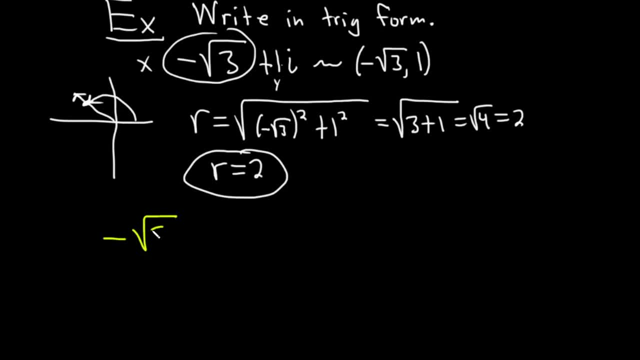 So watch this. So we're going to take our complex number and we're going to set it equal to the polar form. We're going to force it So we know it's r- parentheses- cosine theta plus i sine theta. 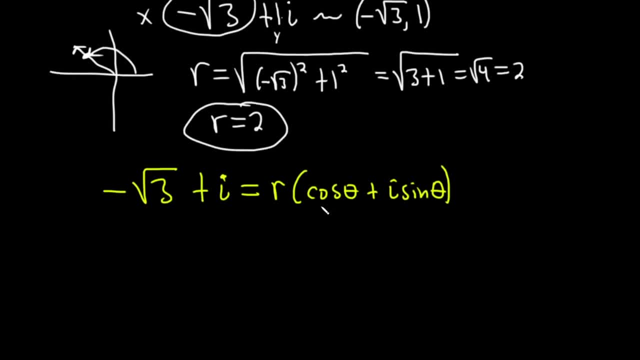 I think this is a much nicer approach than most textbooks, but that's just my opinion. r is equal to 2.. So this is 2 cosine theta plus i sine theta. So this is equal to 2 cosine theta plus 2 i sine theta. 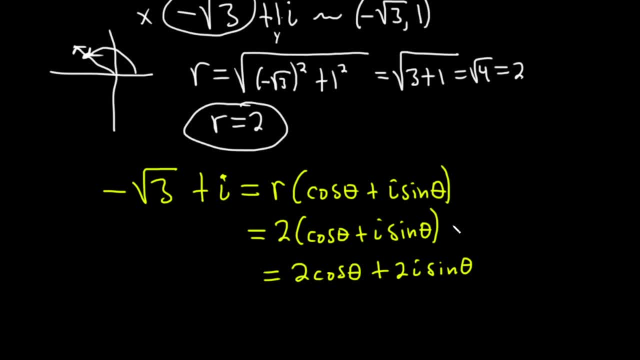 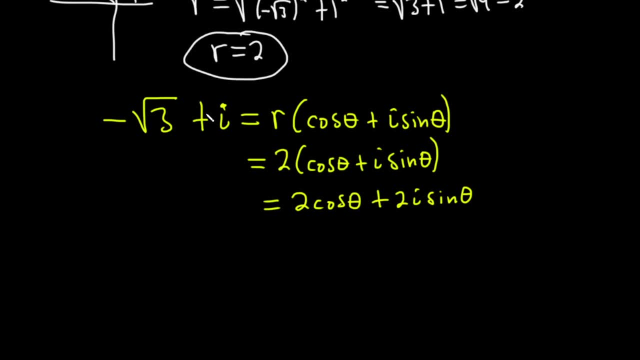 So this is certainly more work than just computing the tangent, But when you do that, you do have to rely on memorization, whereas this relies on just the most basic of mathematics. And now we're going to use a very powerful fact. 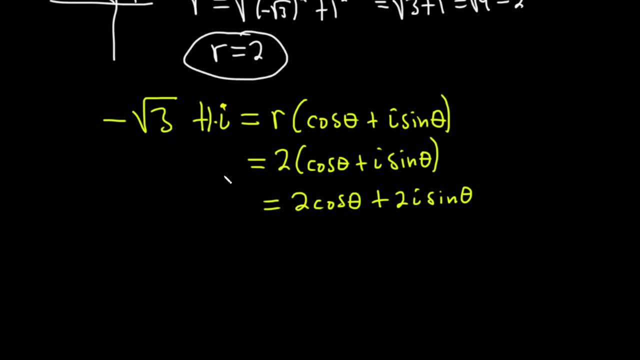 Whenever you have two complex numbers and they're equal, that means you're going to be able to memorize them. So when you have two complex numbers and they're equal, that means they're real parts and they're imaginary parts are equal. 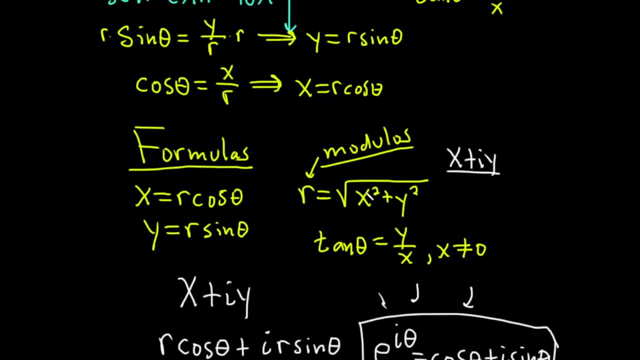 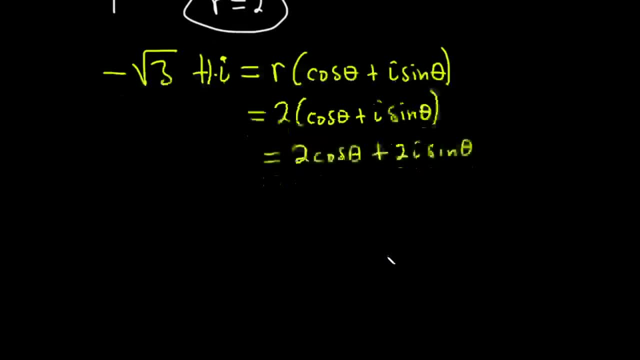 So remember the real part? let me go back up to the top and show you. at the very beginning of the video we mentioned it. The real part here is a and the imaginary part here is b. So down over here the real part is going to be this: 2 cosine theta. 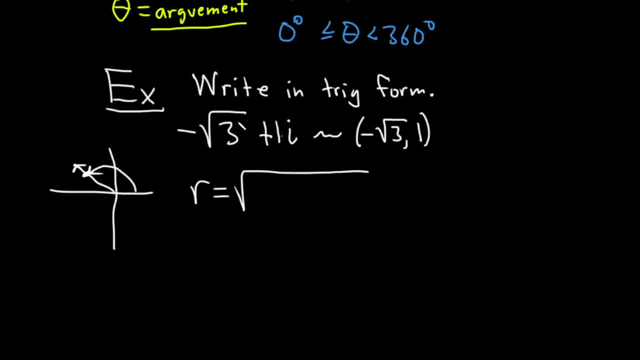 So r is equal to the square root of So x here, by the way, is negative root three. And then y is equal to one. Okay, This will be negative root. three squared plus one squared. This is going to be the square root of. 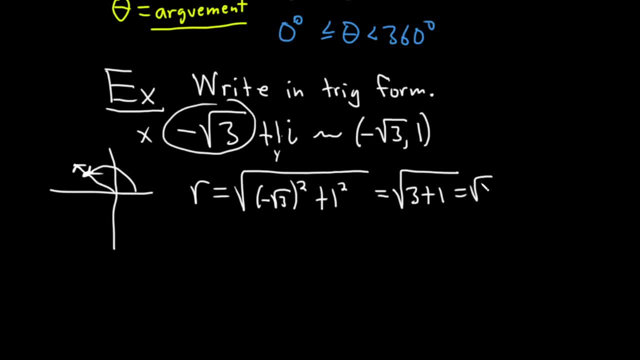 When you square this, you're just going to get three. Square one, you get one. Get the square root of four, so you get two. So r is two, So r is two. Okay, That's the modulus. 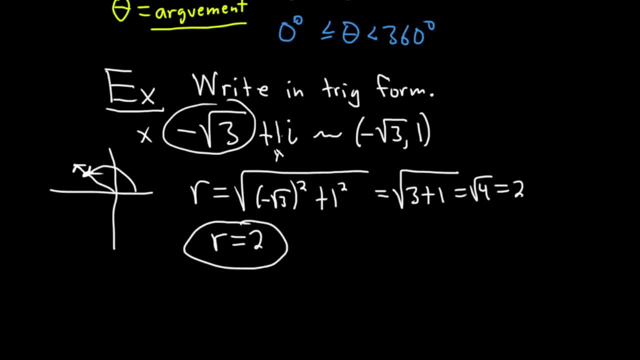 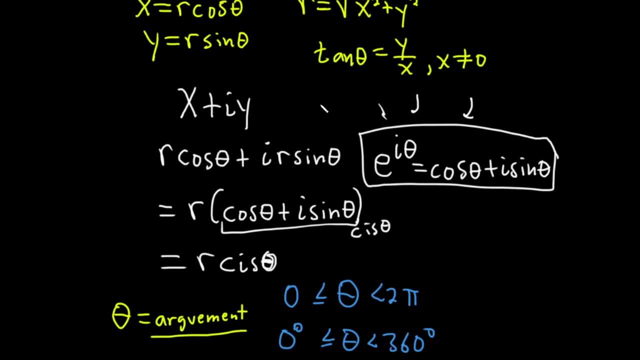 Most people. what they do now is they look at the tangent function and they do. tan of theta equals y over x. You could do that but maybe you don't have you know the trig function values of the tangent function memorized. 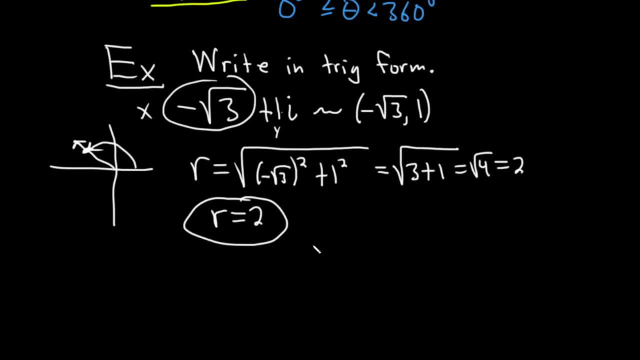 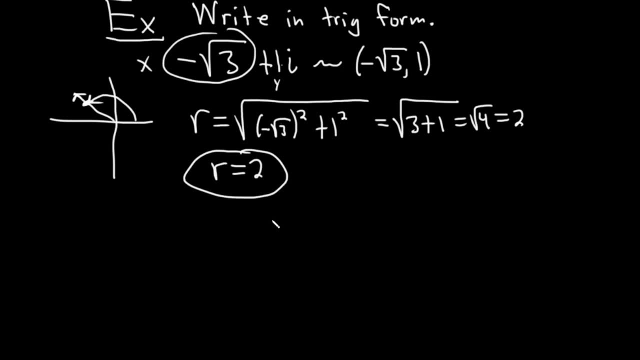 In fact, a lot of people don't, So let's do it another way. that requires minimal memorization. So it's kind of a really interesting method because it kind of shows you where the polar form comes from algebraically. So watch this. 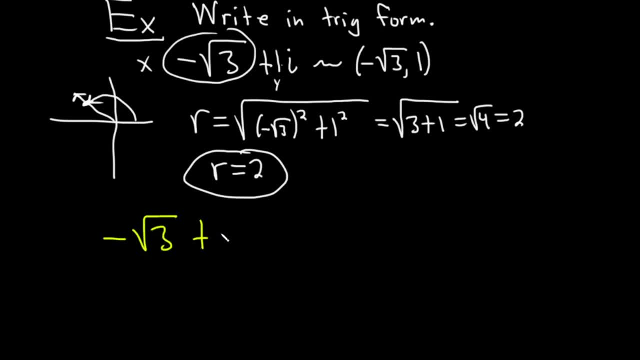 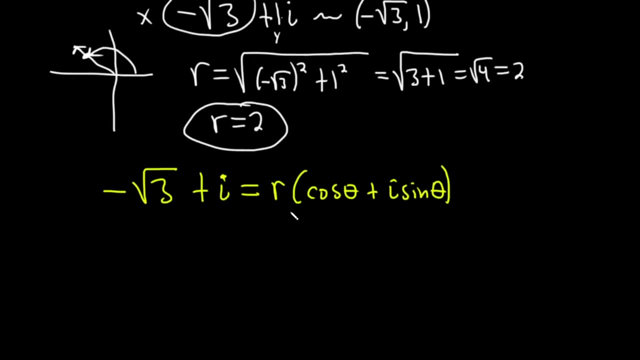 So we're going to take our complex number and we're going to set it equal to the polar form. We're going to force it So we know it's r- parentheses- cosine theta plus i sine theta. I think this is a much nicer approach than most textbooks, but that's just my opinion. 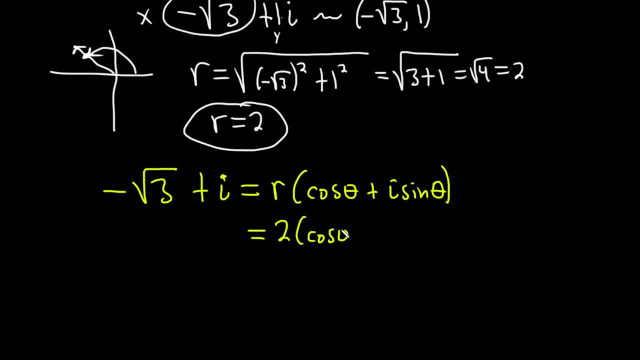 r is equal to two. So this is two cosine theta plus i sine theta. So this is equal to two cosine theta. So this is certainly more work than just computing the tangent. but when you do that you do have to rely on memorization. 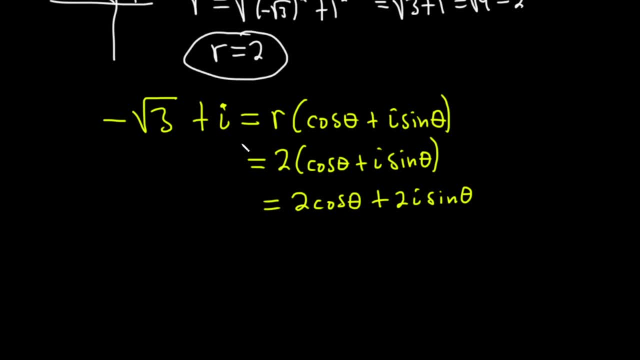 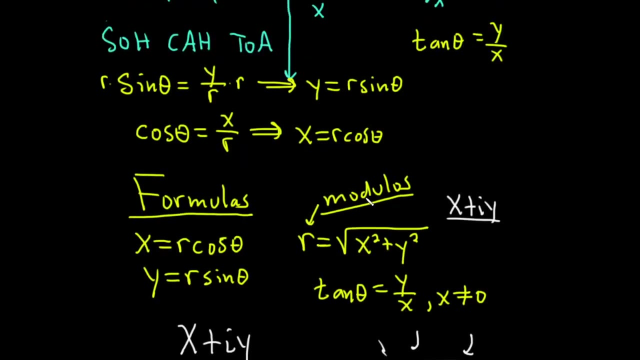 whereas this relies on just the most basic of mathematics. And now we're going to use a very powerful fact: Whenever you have two complex numbers and they're equal, that means the real parts and their imaginary parts are equal. So remember the real part. let me go back up to the top and show you. at the very beginning of the video, we mentioned it. 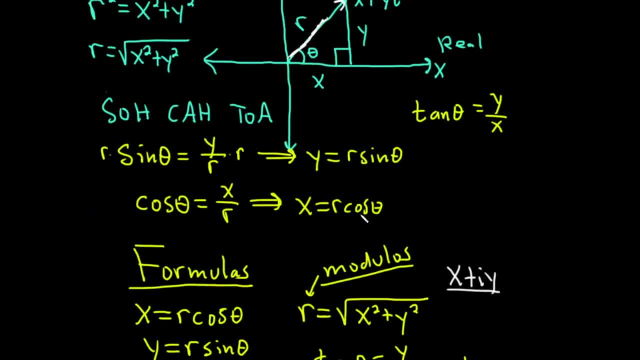 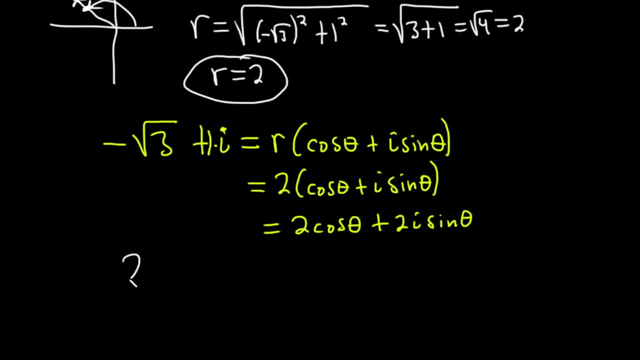 The real part here is equal to the polar form. So down over here the real part is going to be this: two cosine theta. So what you do is you take two cosine theta, right. The real parts must be equal. So this is equal to negative root three. 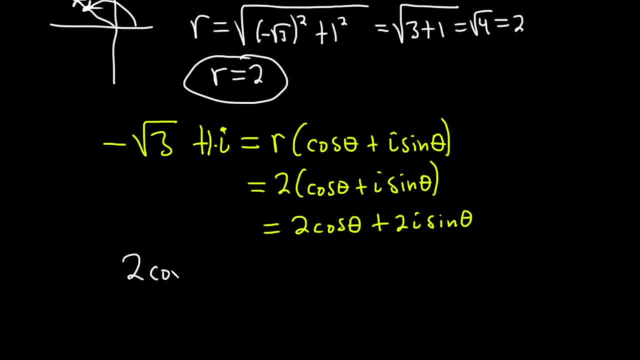 So what you do is you take 2 cosine theta, right, the real parts must be equal. So this is equal to negative root three. Really nice, and that tells you something which we'll come back to. and then the imaginary part. 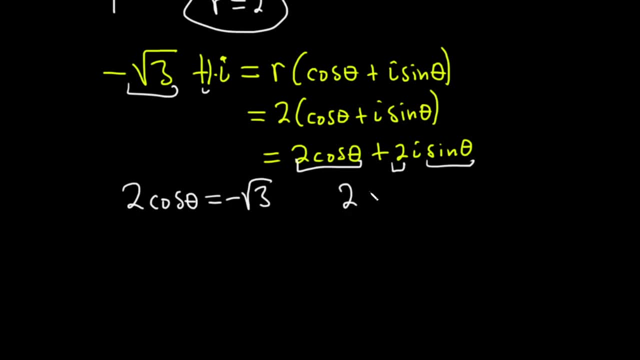 two sine theta is equal to one. so two sine theta equals one. so we have the cosine of theta equals negative root. three over two sine of theta equals one half. and this really tells you the quadrant in some sense, right? it lets you know: oh, hey, i'm in quadrant two. right, because 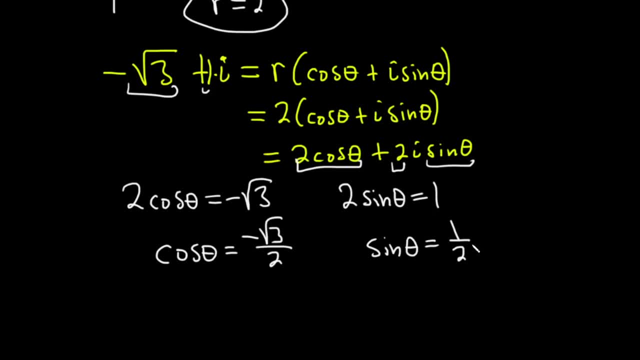 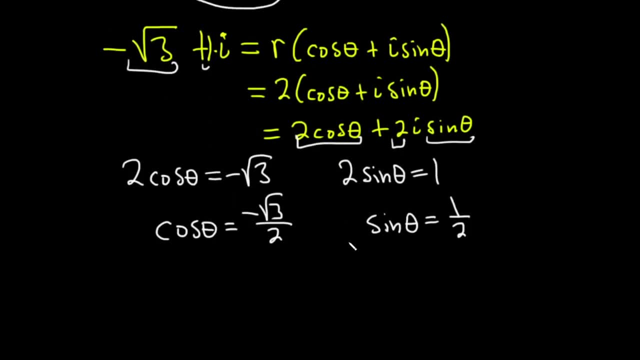 remember, on the unit circle, cosine is the x coordinate, sine is the y coordinate, so it really helps you. so if you forget to draw the picture, for whatever reason, this service is a really good reminder. okay, whereas if you just use the tangent function to um to do this problem, 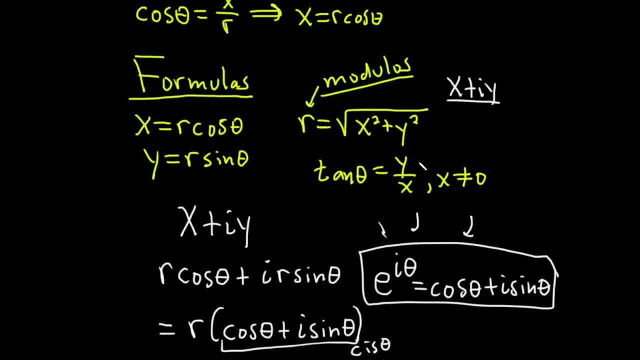 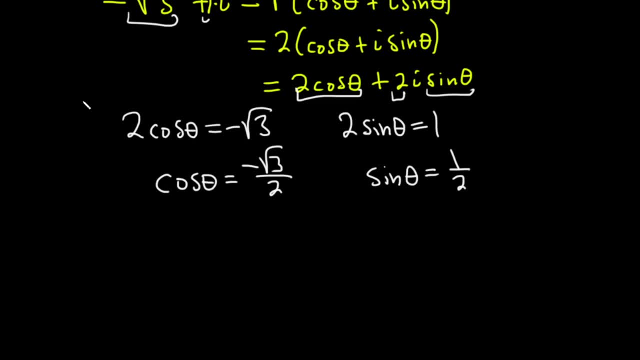 right, you compute tangent of theta equals y over x. you know, if you did that, um, you would have to use some other skills. right, you would have to know some stuff. for example, if you compute tan of theta equals y over x, well, y here was one and x was negative root three. so you have to know, hey. 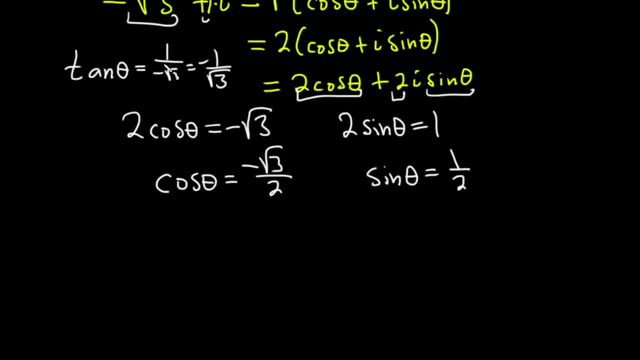 what is theta going to be in this case? so you really have to think about where you are and you also have to think about um. you know ref, it's just a little bit harder for most people, so here this is a little bit easier. um, we know that the, for example. we know, for example, the sine. 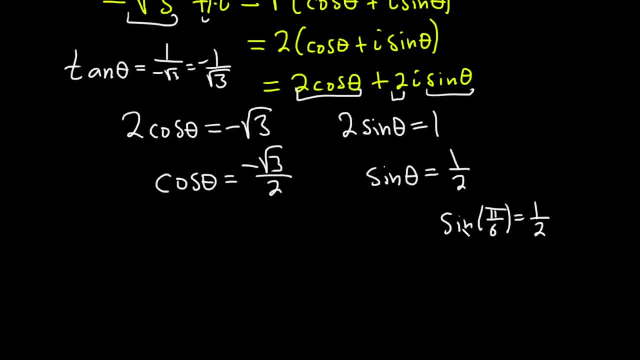 and cosine functions. so we definitely want to have those angles memorized from the first quadrant, in particular pi over three, pi over four and pi over six for the sine and cosine functions. if you know those cold you can do all of these problems. and likewise cosine of pi over six would. 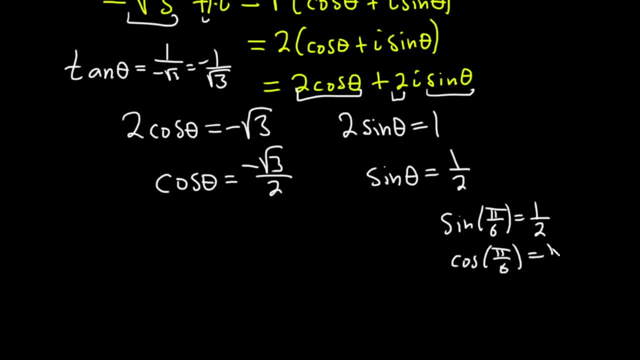 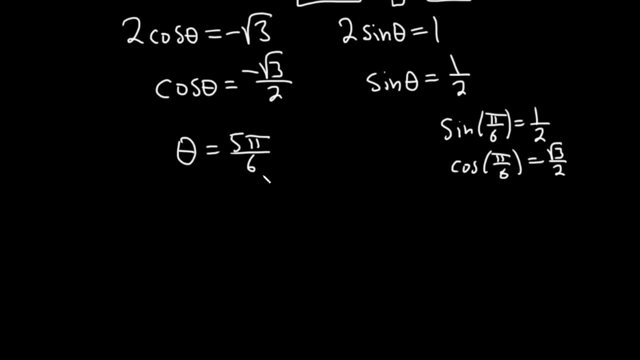 be root three over two, except, um, we are in quadrant two, right? so that's going to be five pi over six. the theta is five pi over six in this case. okay, so, and how do i know that? again, just from the unit circle. here's pi: think of pi as six pi over. 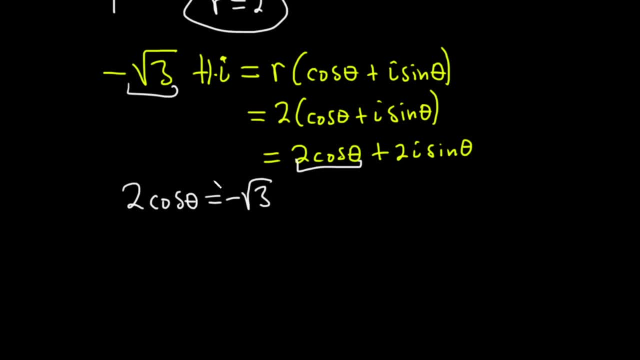 Really nice And that tells you something which we'll come back to. And then the imaginary part: two sine theta is equal to one. So two sine theta equals one. So we have two cosine theta, We have the cosine of theta equals negative root three over two sine of theta equals one half. 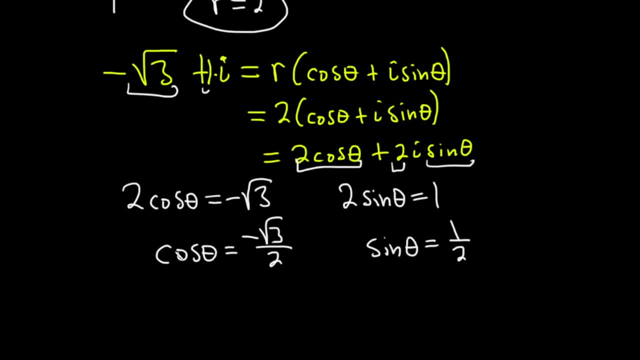 And this really tells you the quadrant in some sense, right. It lets you know, oh hey, I'm in quadrant two, right? Because remember, on the unit circle, cosine is the x-coordinate, sine is the y-coordinate, So it really helps you. 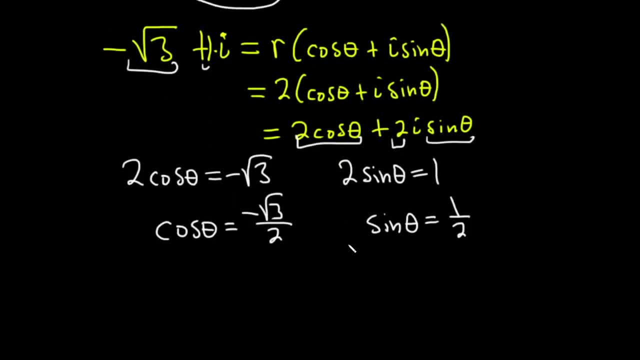 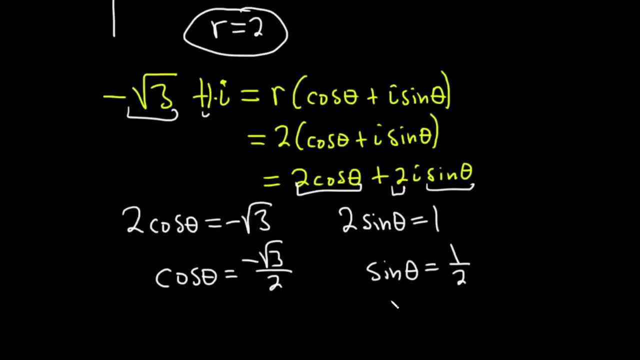 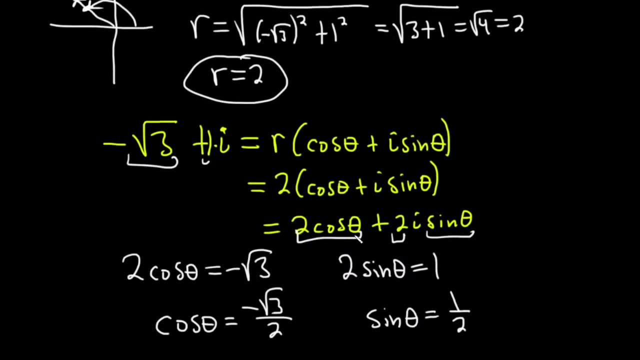 So if you forget to draw the picture, for whatever reason, this serves as a really good reminder, okay. Whereas if you just use the tangent function to do this problem right, You compute: tangent of theta equals y over x. You know, if you did that you would have to use some other skills, right? 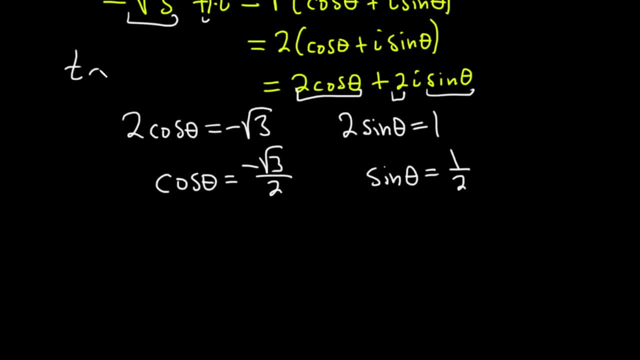 You would have to know some stuff. For example, if you compute tan of theta, equals y over x. well, y here was one and x was negative root three. So you have to know, hey, what is theta going to be in this case? 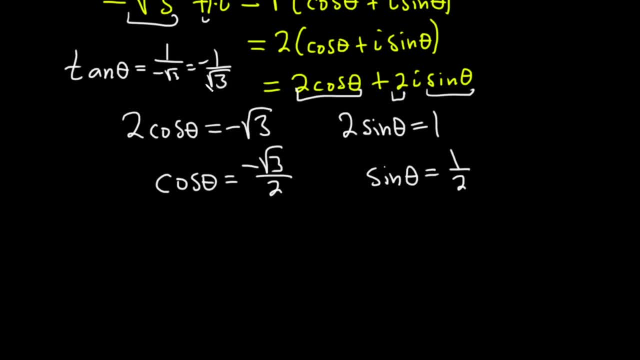 So you really have to think about where you are And you also have to think about. you know it's just a little bit harder for most people, So here this is a little bit easier. We know that the, for example. we know, for example, 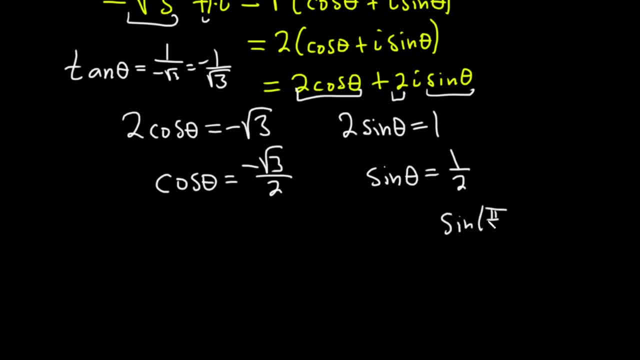 that the sine of pi over six is equal to one half. from memory You definitely want to have those angles memorized from the first quadrant, In particular: pi over three, pi over four and pi over six for the sine and cosine functions. 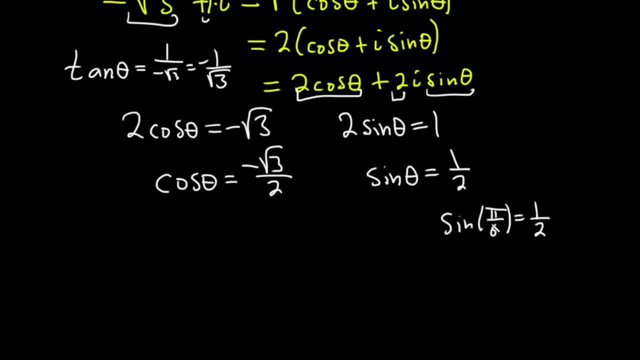 If you know those cold you can do all of these problems. And likewise cosine of pi over six would be root three over two, Except we are in quadrant two right. So that's going to be five pi over six. The theta is five pi over six in this case. 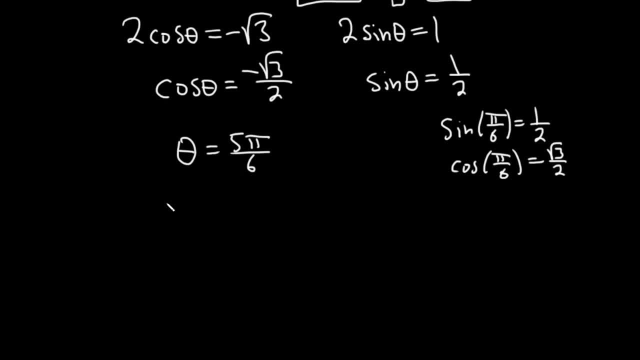 Okay. So, and how do I know that? Again, just from the unit circle. Here's pi. Think of pi as six, pi over six. So the angle that's a multiple of pi over six that lives in this quadrant is pi over six.